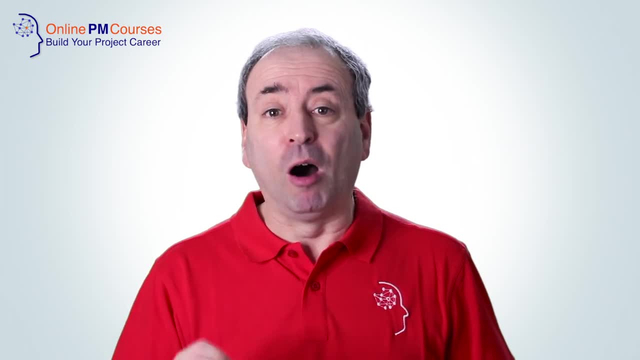 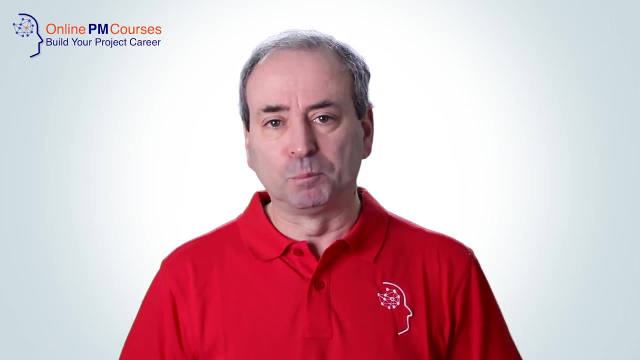 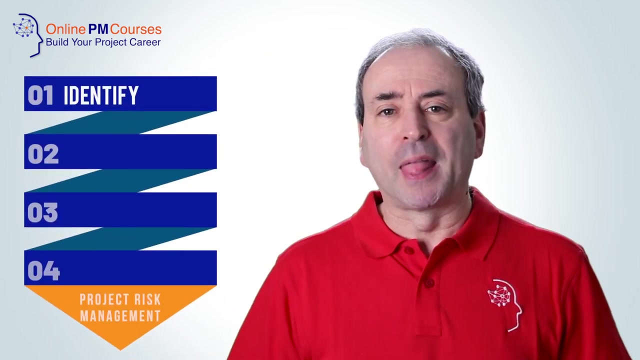 can happen that you're not expecting. Projects are inherently risky, and so we need to manage that risk, to stay in control of our projects, and the basic risk management process has four steps. The first step is to identify the risks, and the best way is always to get a group of people. 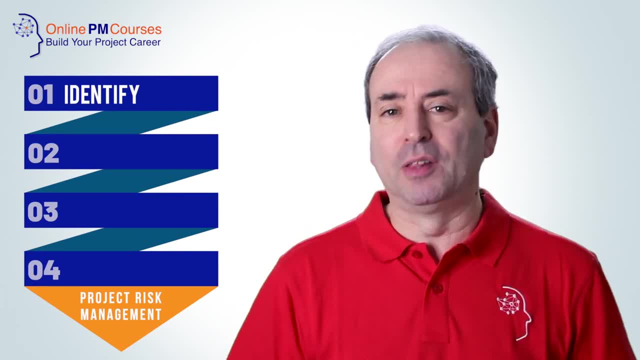 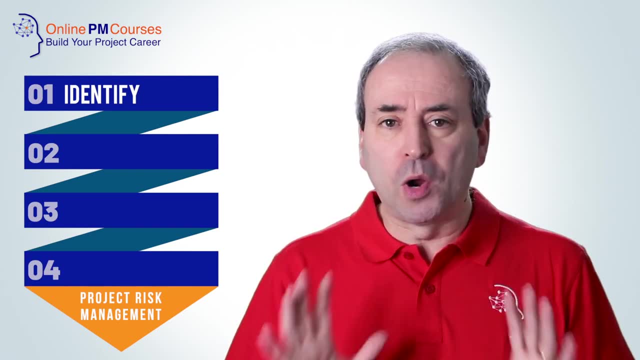 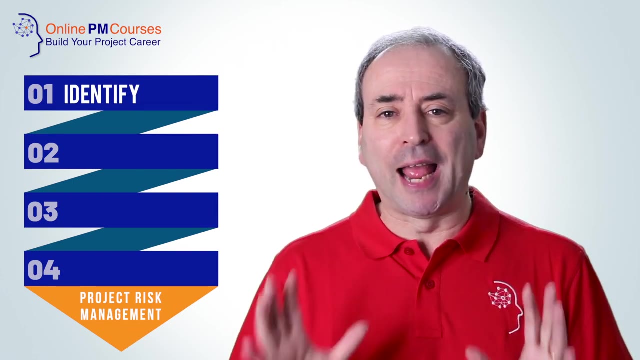 together and just list out everything you can think of that could possibly go wrong. Of course, some of the things you think of are incredibly unlikely, but we'll come to that later. Another good way to identify risks is to look at the different aspects of the project. 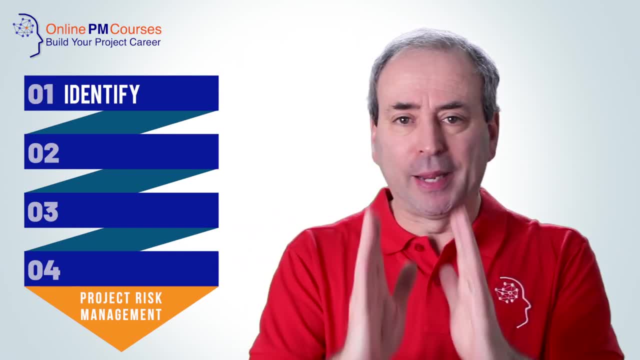 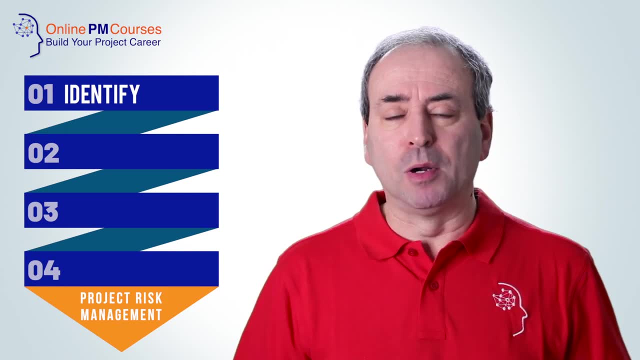 and ask what can go wrong. on a category by category basis, however, you choose to break up your project, And so risk management can start in earnest once you've started to think about the scope of your project, and you can go to a greater level of. 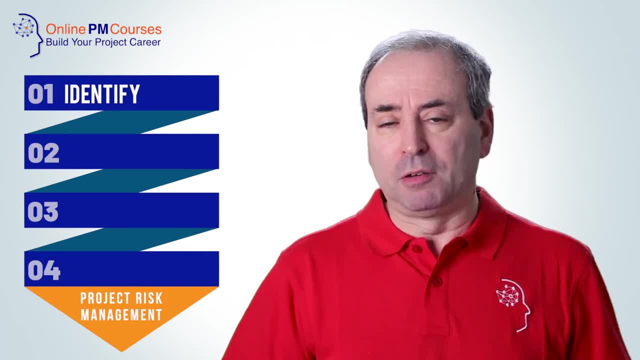 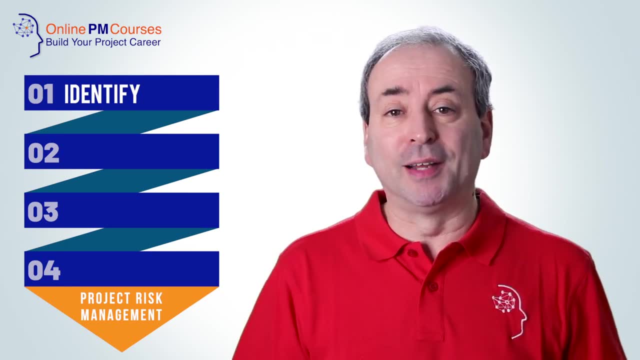 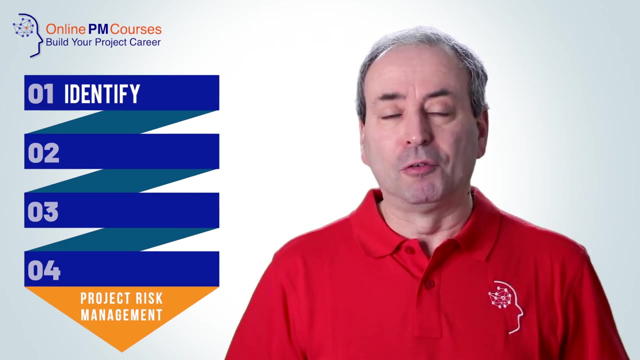 risk once you've got a work breakdown structure. Another great approach is, as you move through your career from one project to another, keep a record of all the risks that are identified in each project, and that way you'll have a master list of risks which you can draw down on for identifying. 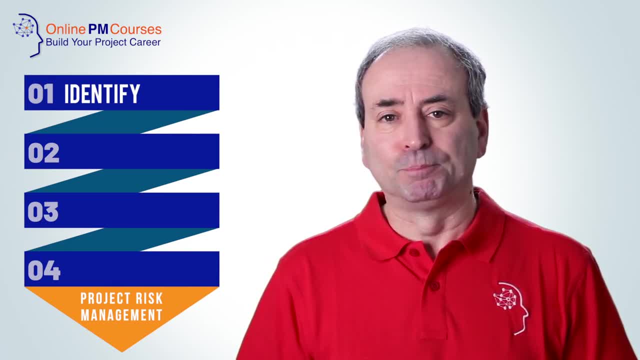 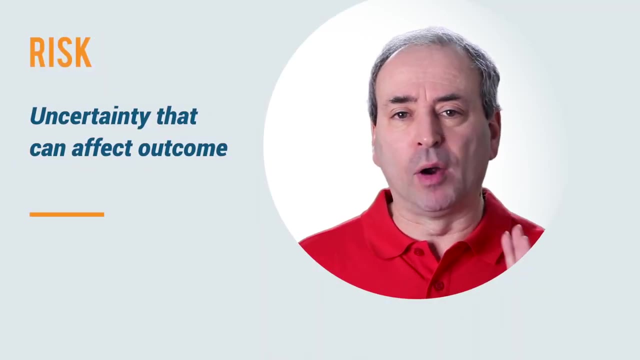 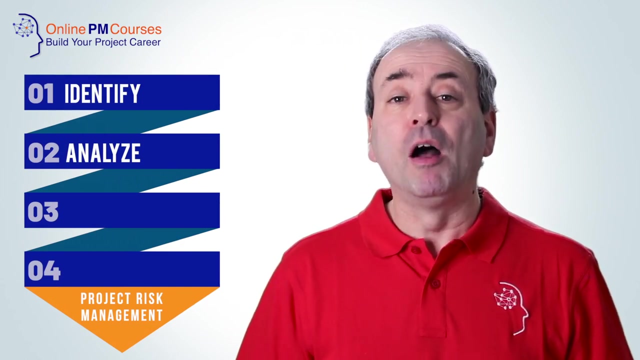 potential risks for each new project. Once you've identified your risks, the next step is to understand them, to analyse those risks. Now, the definition of a risk is uncertainty that can affect outcome. Therefore, the two principal components of a risk are the likelihood with which it might happen. 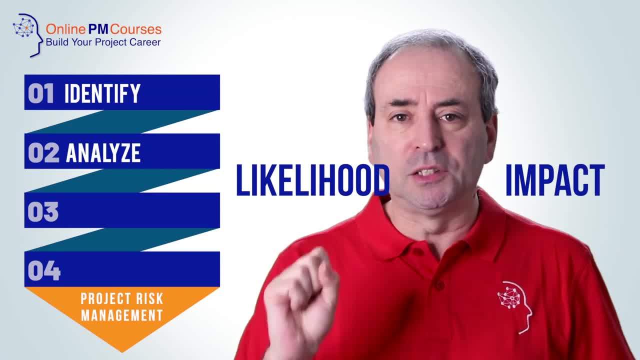 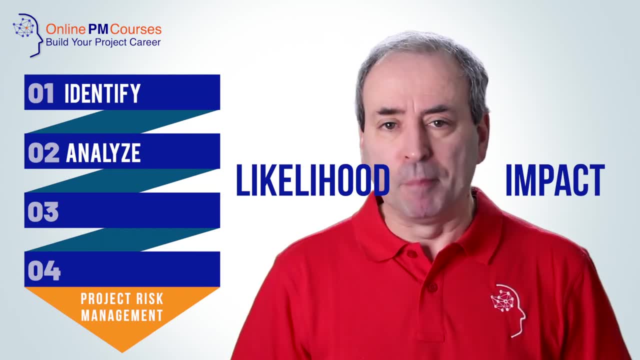 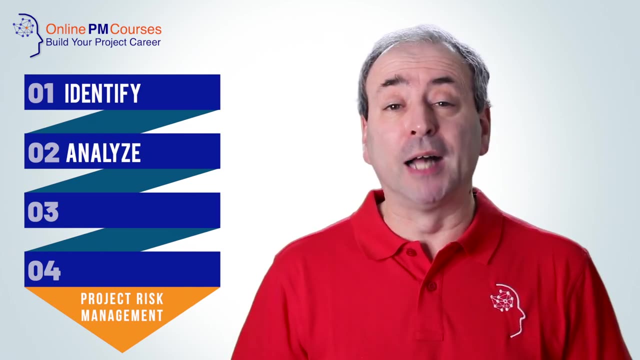 and the impact it will have if it does. The uncertainty is measured by likelihood and the effect on the project is measured by the impact. There are other things we can bring into our analysis if we're taking on risk management at an advanced level, like proximity. However, for most of us, 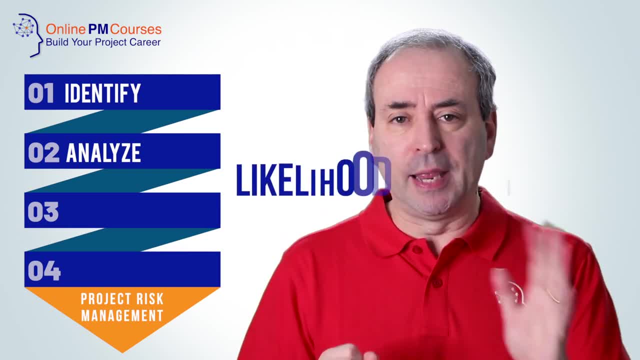 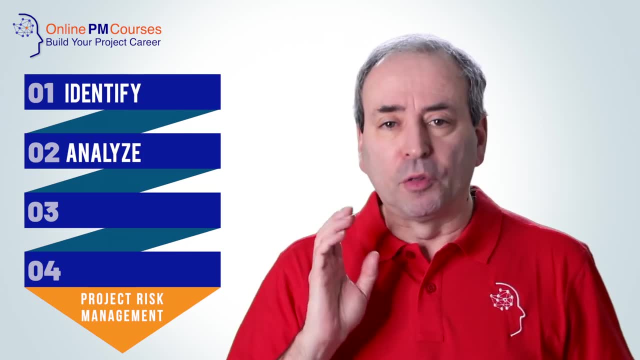 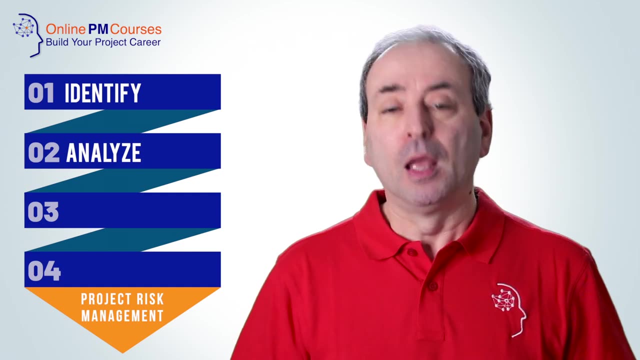 for most projects. estimating the likelihood and the impact of our risks is the key to good risk analysis. Now, when you're thinking about likelihood for your risks, my key piece of advice is: keep it simple, Because if you're thinking about risk management at an advanced level, you're going to have to be very careful about what you're doing. If you're thinking about risk management at an advanced level, you're going to have to be very careful about what you're doing. If you're thinking about risk management at an advanced level, you're going to have to be very careful about what you're doing. 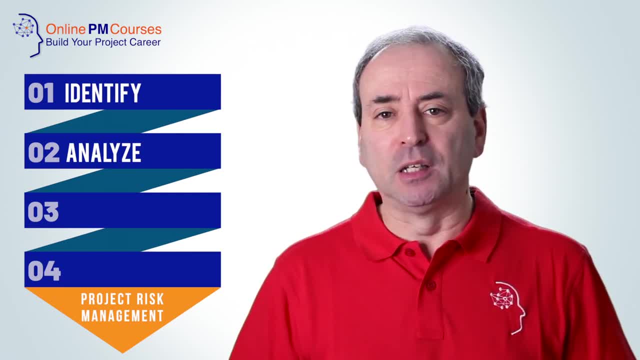 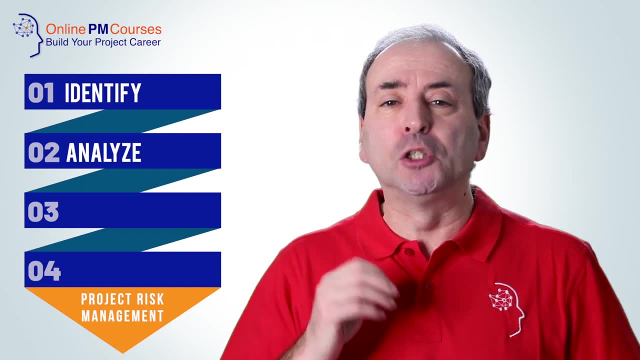 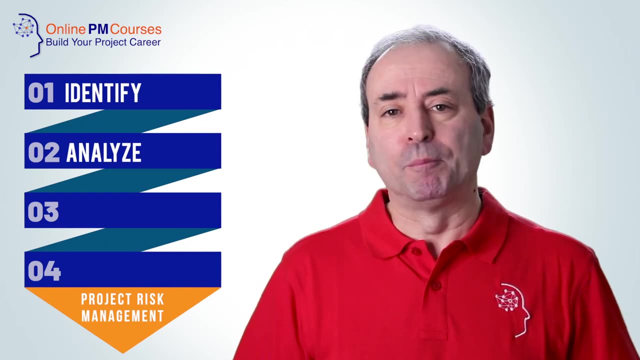 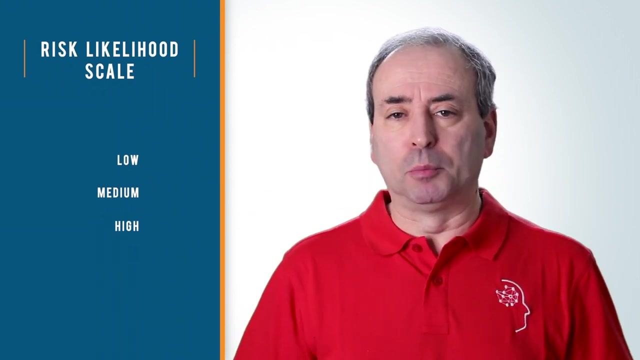 human beings are rubbish at estimating the likelihood of uncertain events, and the consequence of that is that if you try to be too precise, too specific about the likelihood of your estimates, then they're likely to be rubbish. a simple scale of low, medium and high. or, if you want a little bit more precision, very low, low, medium, high and very high. 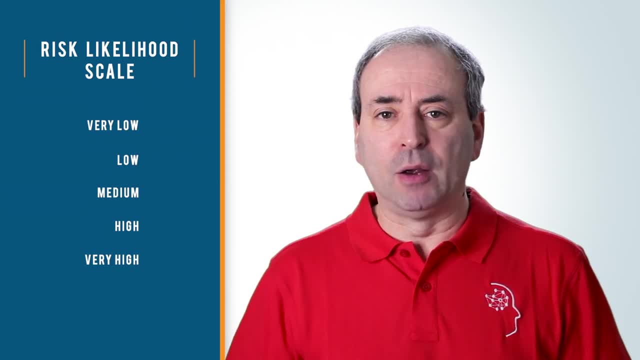 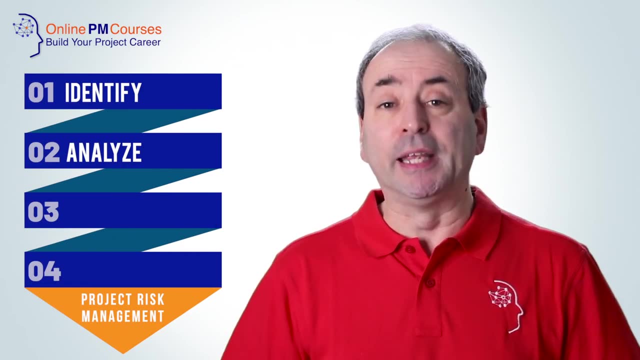 is all you need as a scale for the likelihood of your risks, for the impact. you can use a more sophisticated scale if you choose. the first thing to think about is: what do you really care about? do you care about the impact of risks on your budget? because if that's the case, then you may have a. 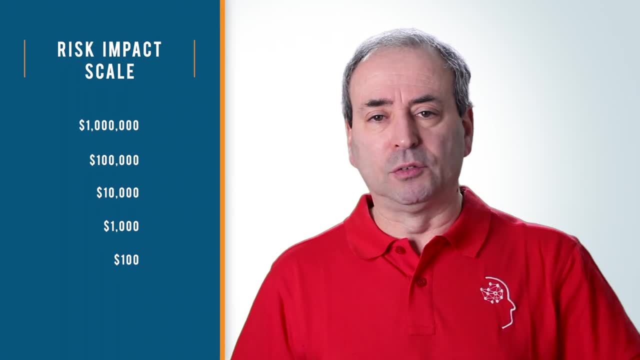 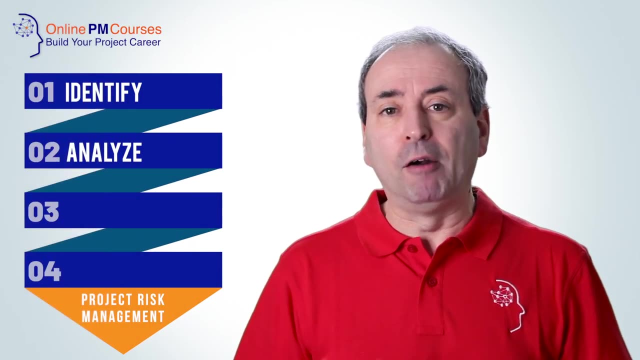 scale of hundreds of dollars, thousands of dollars, tens of thousands of dollars, hundreds of thousands of dollars and even millions of dollars. or you may care about the schedule effect of a risk. what will it do to the delivery date, in which case your impact scale might be days, weeks, months, quarters or years? 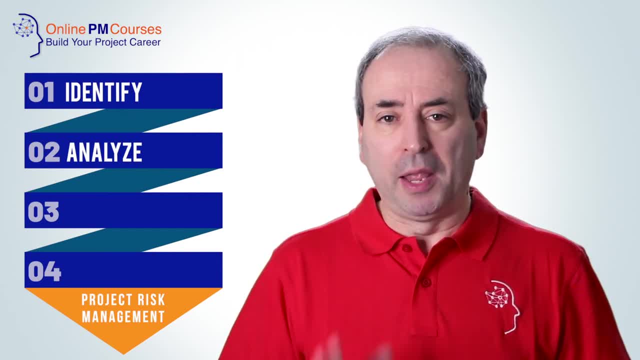 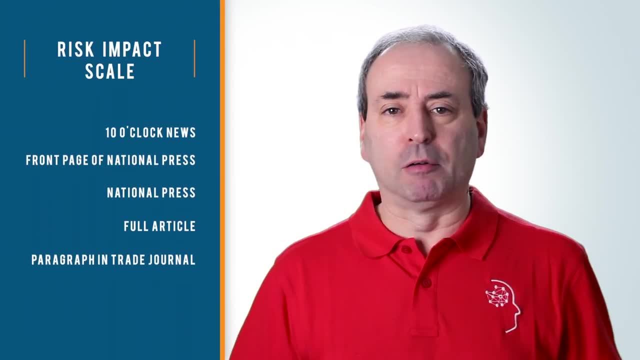 you might be interested in the reputational effects. if something goes wrong, how will it affect our reputation? will we see a small paragraph in a trade journal or a local paper, or will we see a full article? or will that article make its way through to the national press or will it get onto the front? 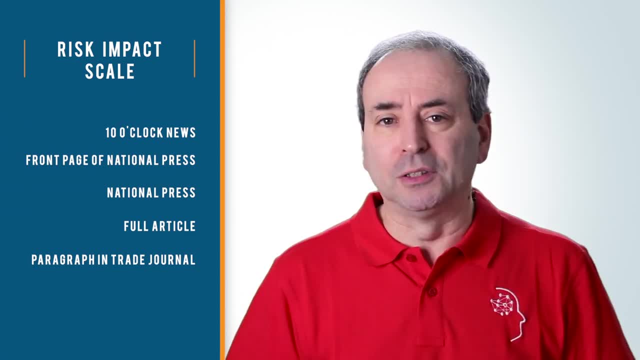 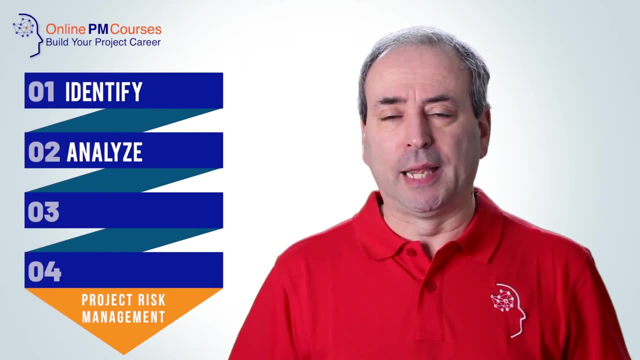 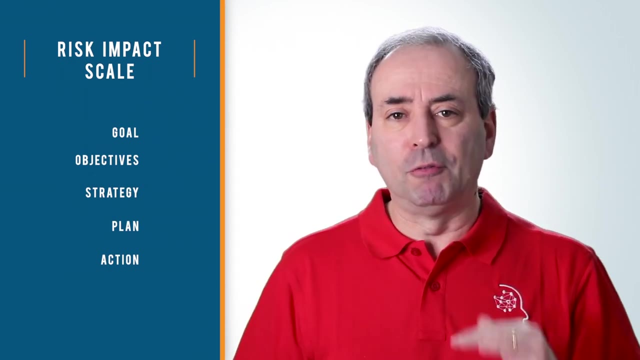 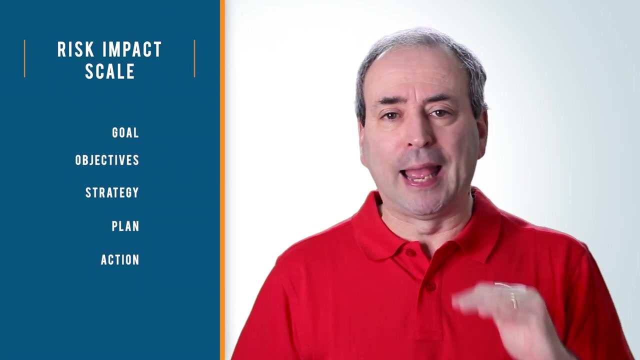 page of the national press, or will it dominate the 10 o'clock news for day after day? but for most of us, a simple scale is to first think about the smallest level of impact being one that requires some form of corrective action. a greater impact may need you to think about a new plan. 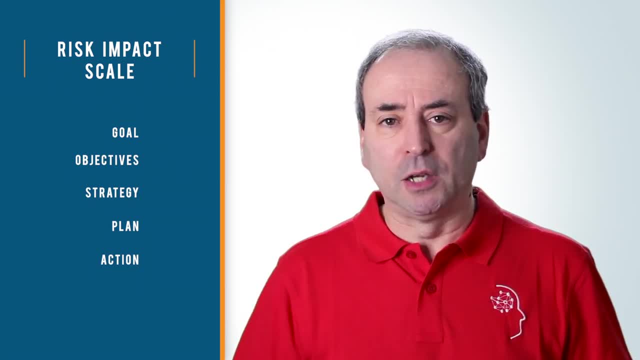 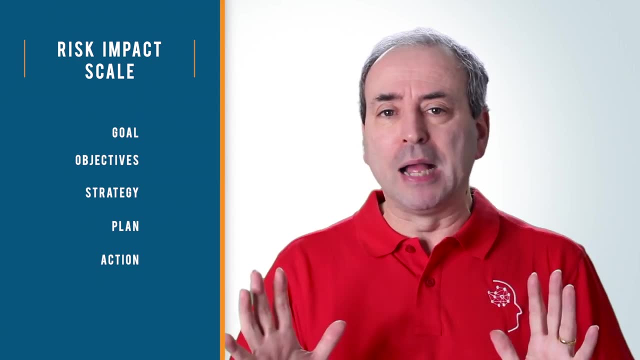 for how you're going to deliver that part of the project, or you may need a whole new strategy for how you're going to deliver the whole project, or it may be worse than that, and no amount of re-planning and new strategies will allow you to achieve all of your objectives. one: 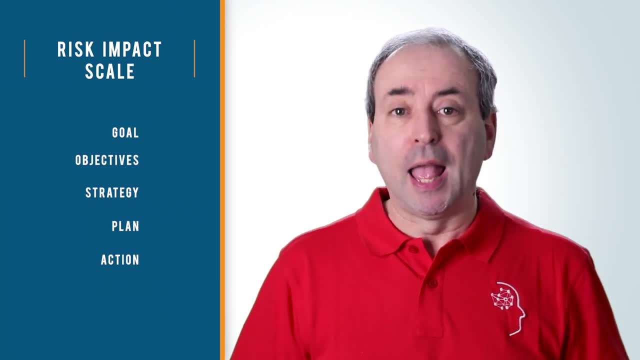 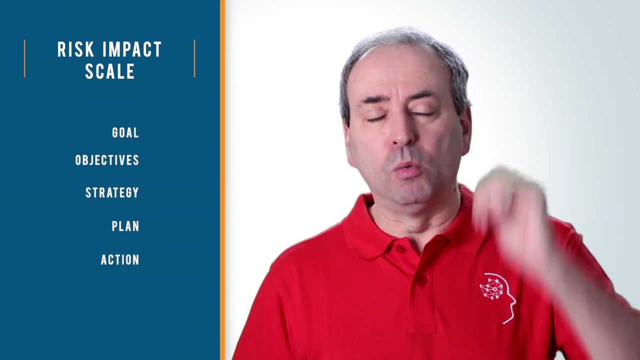 or more of your objectives will be compromised if this risk occurs. and, of course, the greatest level of risk that you should be managing without highly specialized experience is the risk that the project will fail. the goal of your project is compromised. yes, of course there are higher impacts. 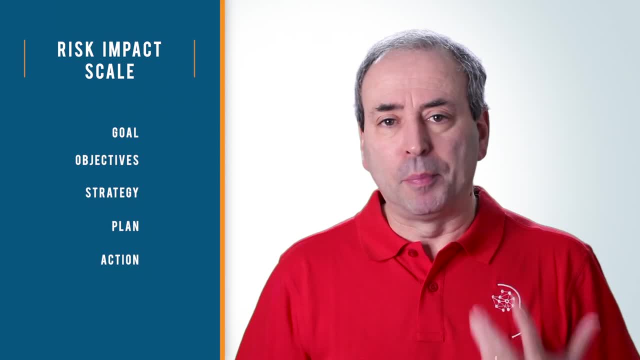 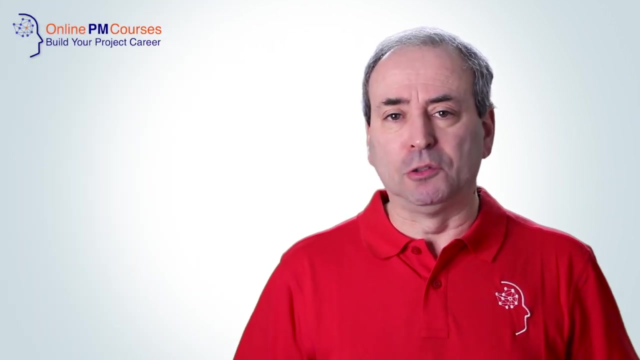 than that, people being hurt or the reputation of your organization being permanently tarnished. but of course, if those are real risks, you need to bring in real experts to help you manage them. now, once you've analyzed your risks, you can then triage them by looking at where they appear on a 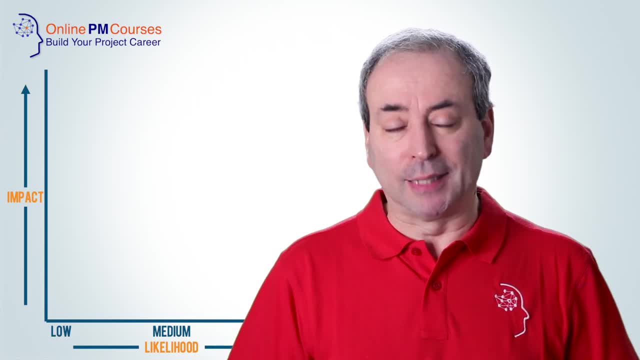 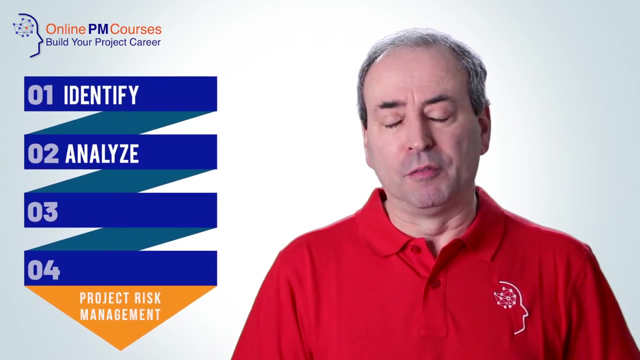 simple graph of likelihood versus impact and of course, the further up towards the top right hand corner that they appear, then the more serious that risk is and the more strategies you will need to manage your risk. so step three of our risk management process is to put together a 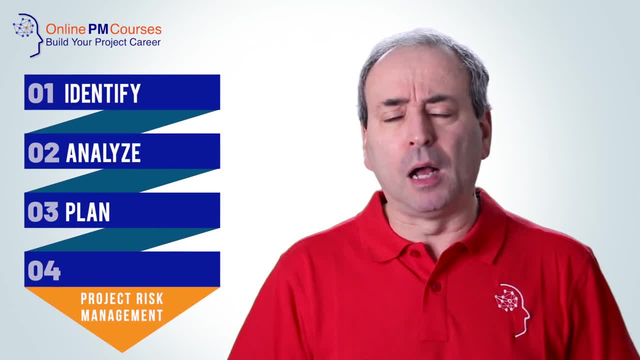 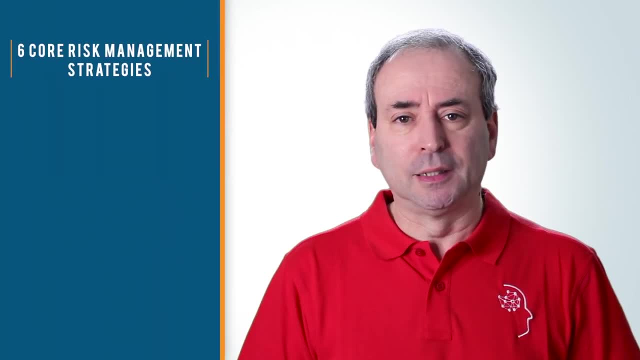 plan for how you will handle that risk, and we build our plans from a number of component strategies, and the six core strategies that i always build my plans from are: firstly, to see if you can do anything to remove the risk entirely. this is the gold standard, but on many projects it for many risks. 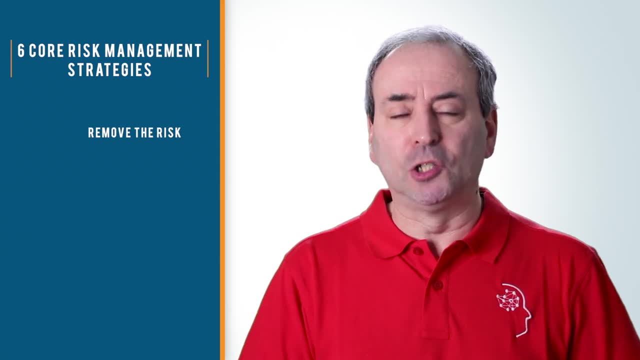 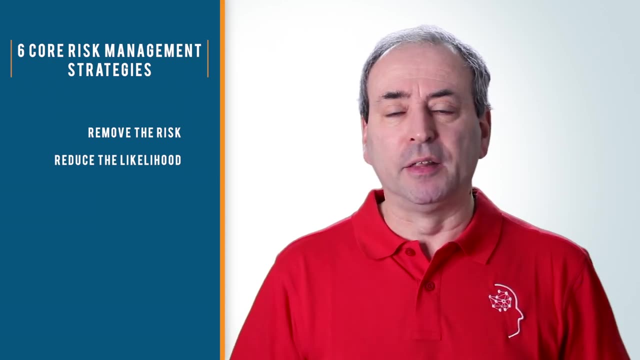 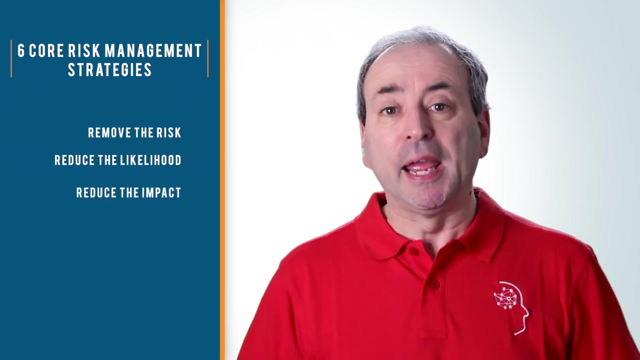 it is not possible to remove the risk entirely, but if you can, you should do so. the second strategy is to reduce the likelihood, to make it less likely that that risk will materialize. strategy number three is to reduce the impact of the risk. if it happens, then what can we do to make? 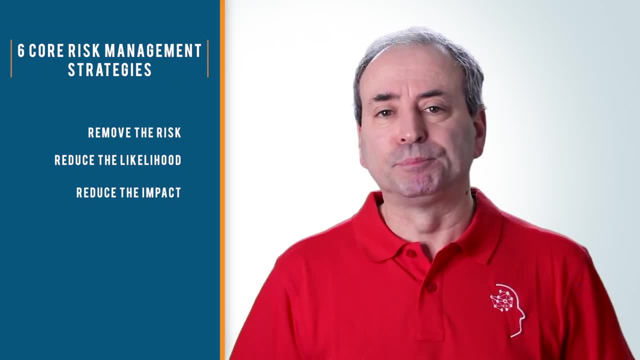 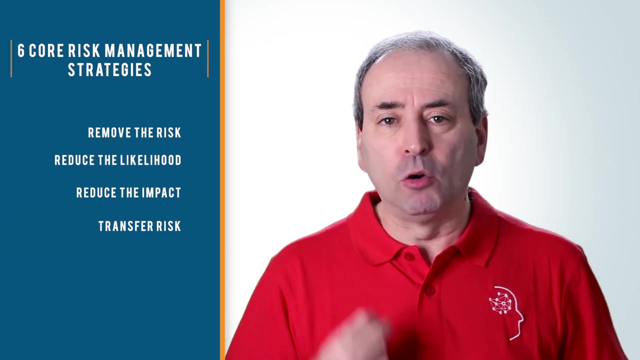 it less severe, less serious. fourthly, we could transfer some or all of that risk to a third party. the obvious example is insurance. but remember, every time you enter into a contract for professional services of one form or another, you are transferring some of that risk to the other party and using the contract to 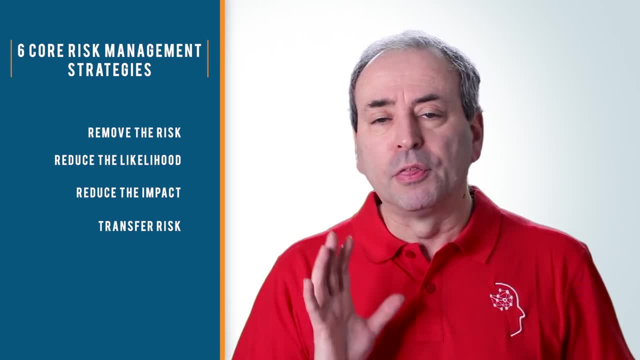 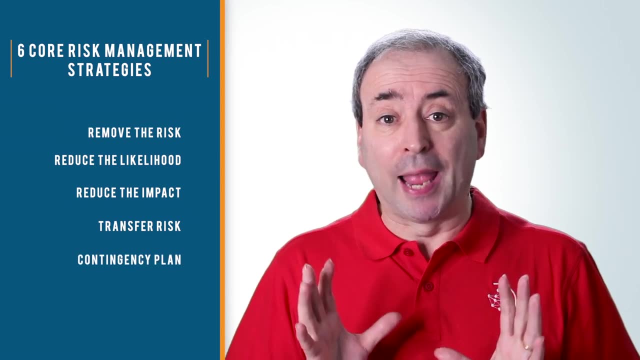 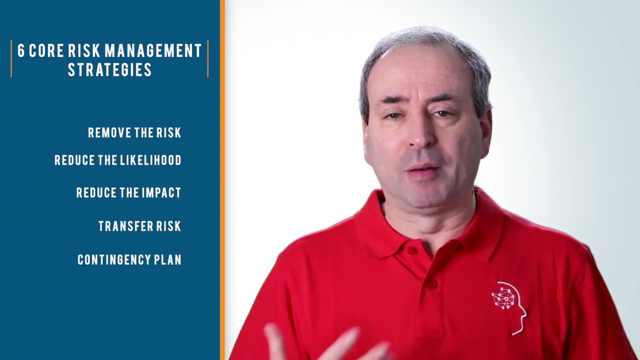 enforce that transfer. the fifth approach is to accept that the risk may happen and to build a contingency plan so that you can handle that risk should it materialize. a plan B: this is about having the resources and the preparedness to deal with the outcome should the risk occur. 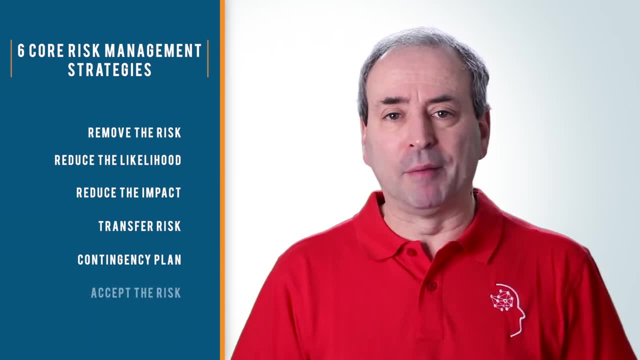 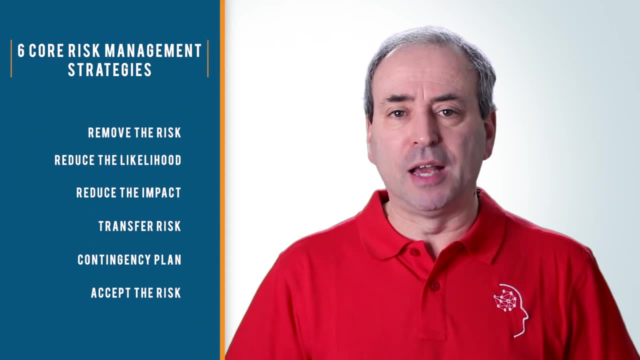 and, of course, the sixth strategy is to accept the risk. if the level of threat is small enough and you consider that none of the other strategies offers a cost-effective solution for reducing the risk, then it's totally appropriate to accept the risk and accept that, if it does occur, you'll need to do something. 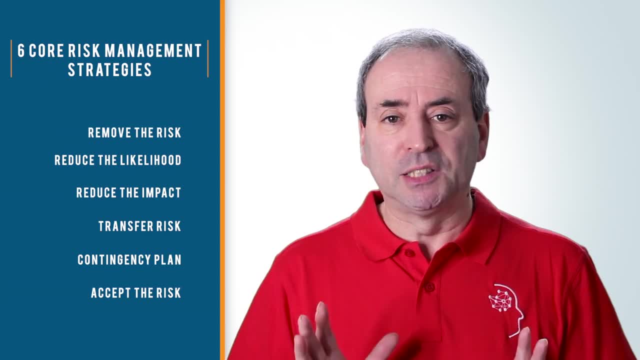 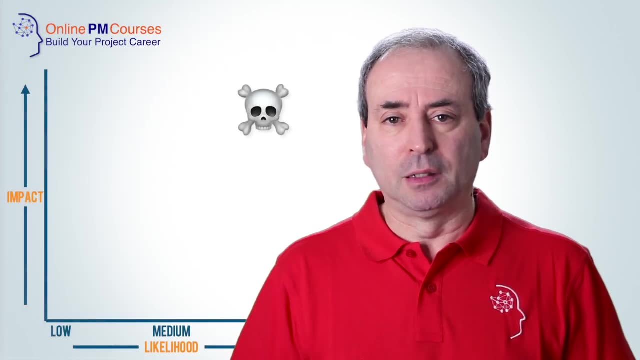 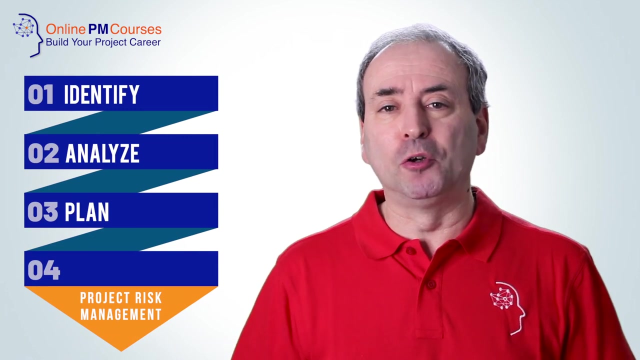 about it, but hopefully it will not be a very serious risk because otherwise you will have implemented one or more strategies and clearly, for the highest likelihood and impact risks to the top right, you'll need a whole basket of strategies to handle them. and finally, the fourth stage of risk management is, of course, to put your 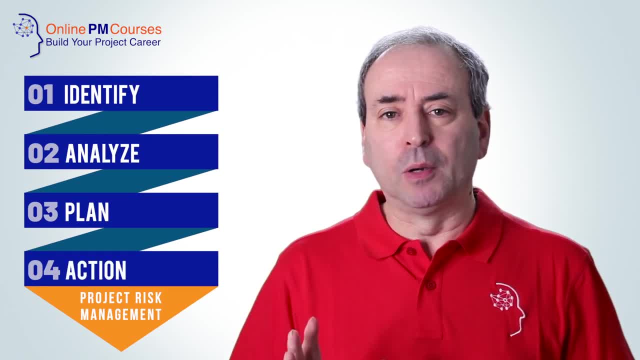 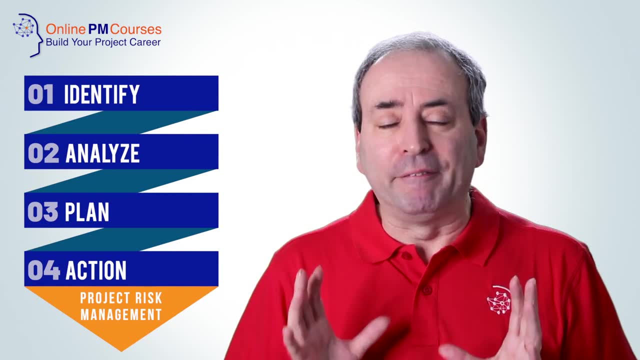 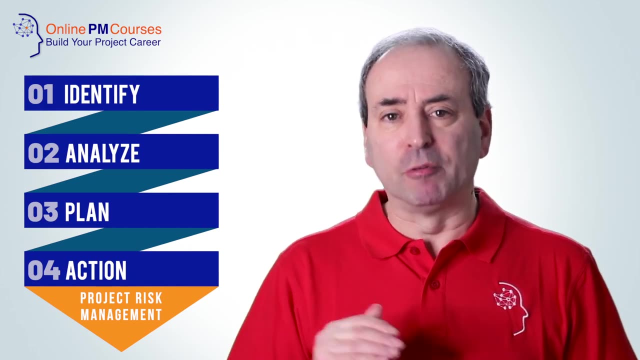 plans into action and, hopefully, you will have documented your risks and your plans on a risk register which is, if anything, the one single most important project management document that you will have. that risk register becomes part of your audit trail and therefore a document of governance, but it's also a 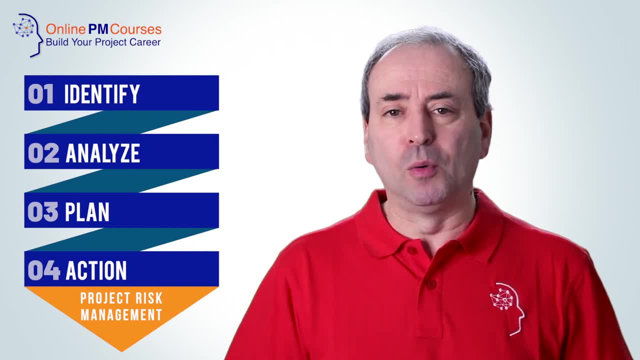 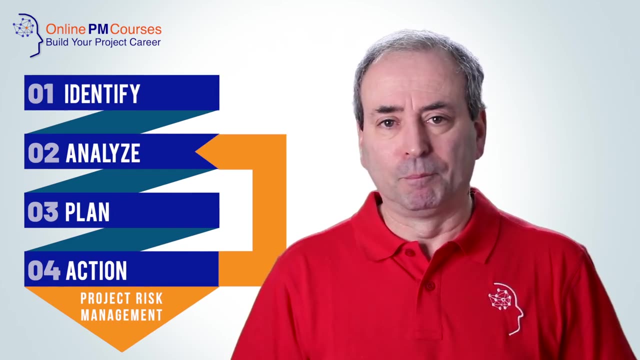 management tool that allows you to track what you are doing and to keep an eye on your risks. and, of course, every time you take an action, you can then record that action on your risk register and monitor the impact it has on your risks if the action doesn't satisfactorily reduce the risk. 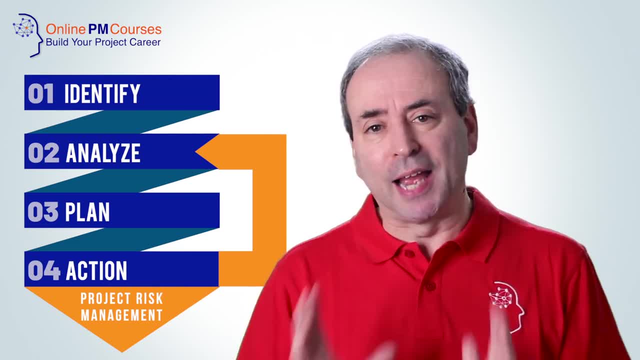 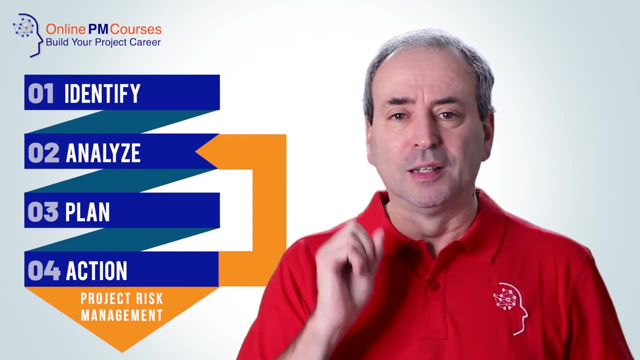 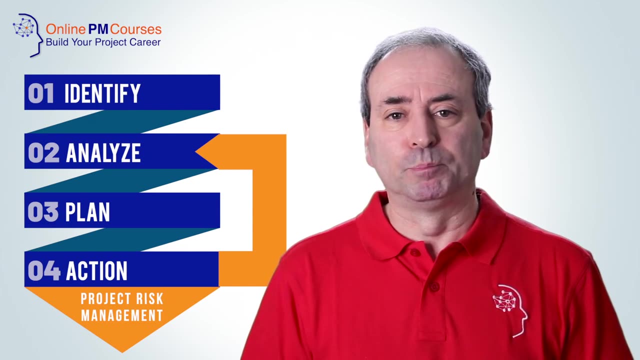 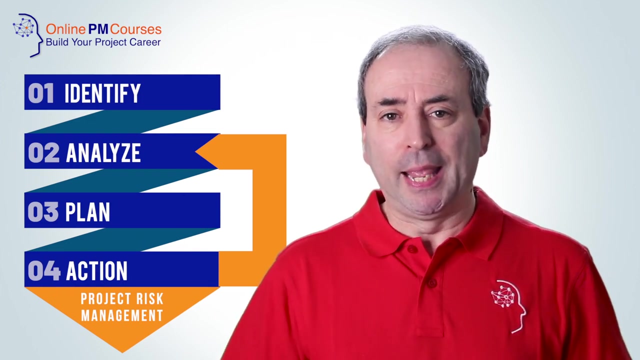 then analyze why not come up with an additional plan and take further action. and that's the cycle of success: understand the situation, put together a plan, take action and review where you are and understand the outcome. so risk management is a simple four-step process. it's supported.